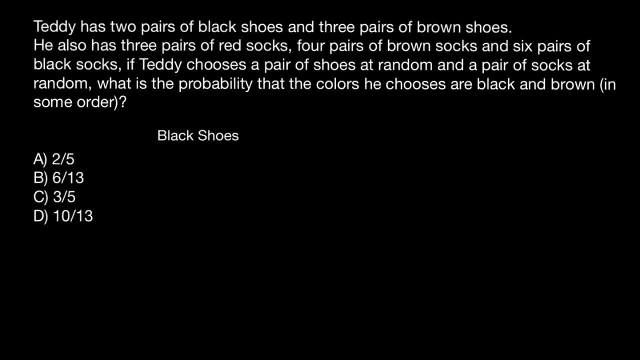 So basically that means that Teddy can choose black shoes and brown socks. We have to find probability of this event, Another variant how Teddy can choose brown and black if he choose brown shoes and black socks. So this is second variant how he can choose black and brown in any order. 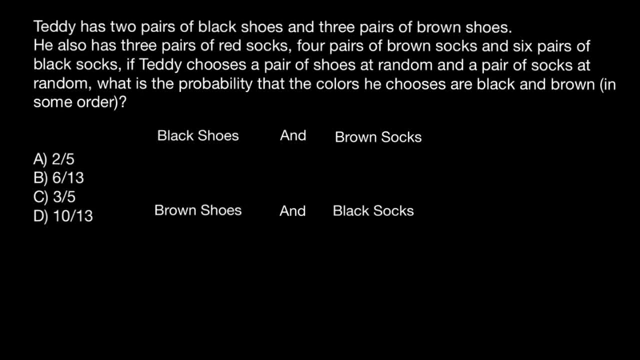 What is the probability that Teddy choose black shoes? So black shoes he has two pairs and three pairs of brown shoes. So total number of shoes he has five And two of them are black. So the probability that he is going to choose black shoes is going to be. 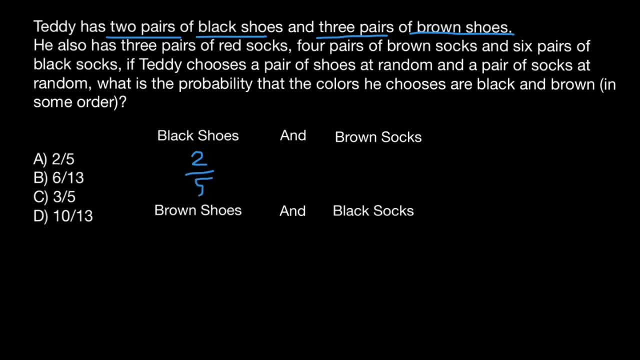 two out of five. That means that probability that he is going to choose brown shoes is going to be three out of five. Three out of five. Now let's find probability for him to choose brown socks or black socks. So he also has three pairs of red socks, four pairs. So let me underline: 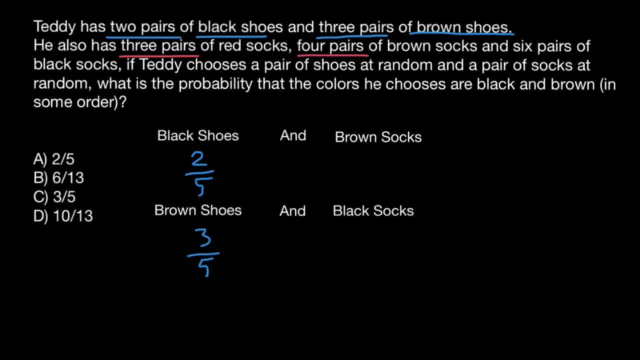 So three pairs of red socks, four pairs of brown socks and six pairs of black socks. So total number is 13.. What is the probability for him to choose, for example, brown Brown socks? it's going to be four, So four out of 13 is probability for him to choose brown socks. 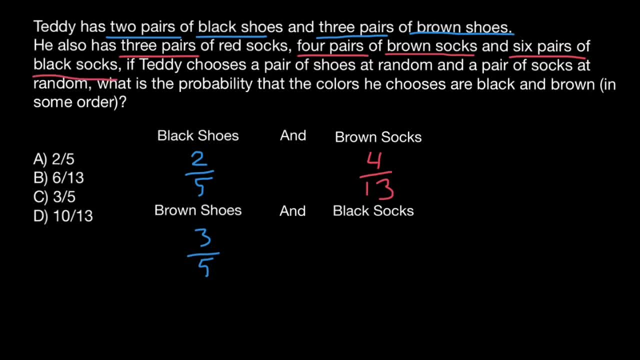 And six pairs of black socks. So 13 out of 13 is probability for him to choose brown socks. That means six out of 13 is a probability for him to choose black socks. Now we have to understand what we should do next. Should we add these probabilities or multiply them? 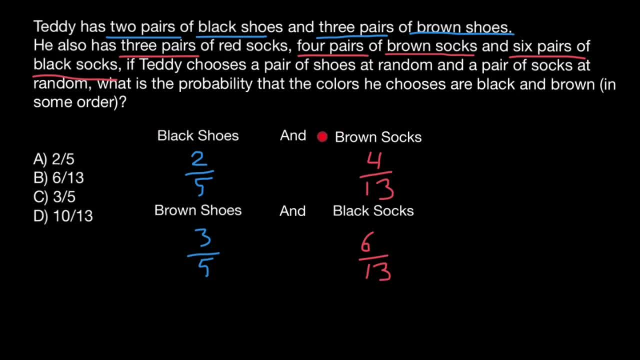 When we have two independent probabilities which we connect with the word and we should use a product rule, We have to multiply such probabilities. Here we also have two probabilities which we connect with the word and So we have to multiply this independent probabilities. So probability of him choosing black shoes. 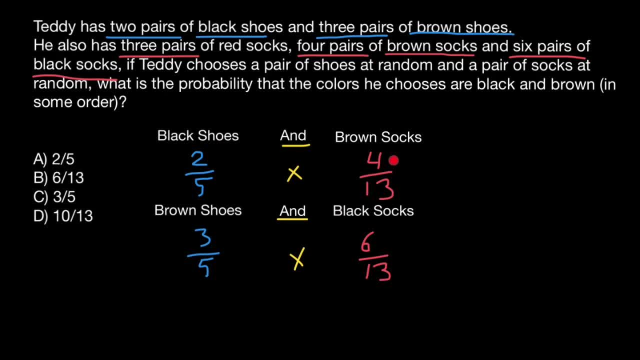 and brown socks. We have to multiply this: two independent probabilities. The same true for brown shoes and black socks. So here we are going to get eight over 65. This is going to be probability for Teddy to choose black shoes and brown socks. 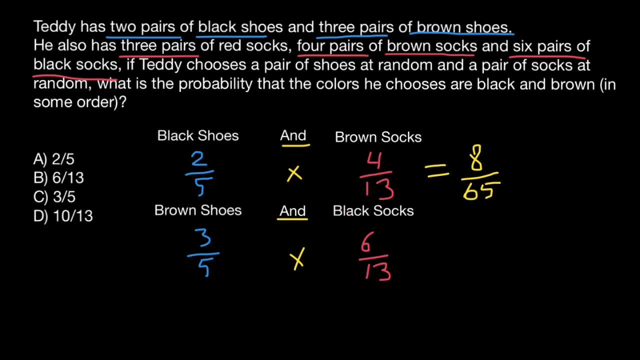 probability for him to choose brown shoes and black socks would be so 3 times 6, 18, 18, over again 65. now we have probability for Teddy to choose this variant or this variant of the colors. both of them meet our requirements, requirements of our problem. in this case, we also can say what is the probability. 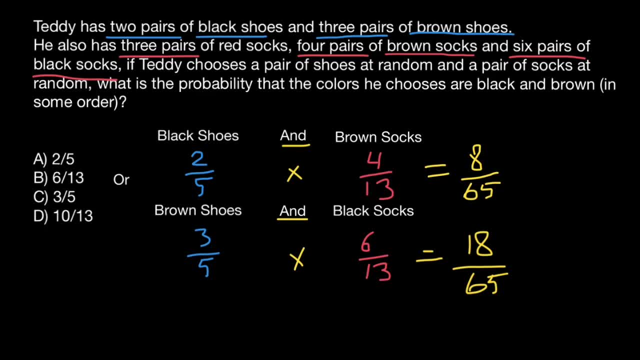 for him to choose this set of events or this set of events. if we connect two probabilities by the word, or we should use a rule of addition, we have to add such probabilities. so that means that we have to add 8 over 65, 25 plus 18 over 65. as you see, both these variants meet requirements of our 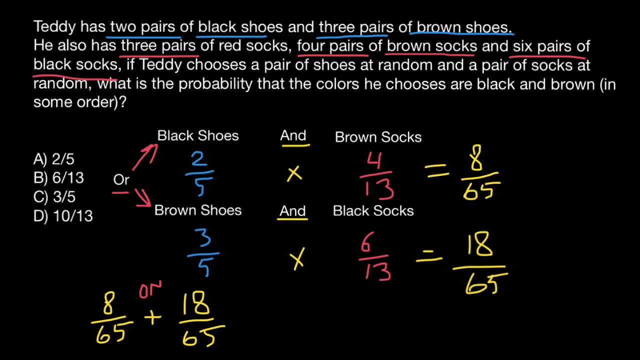 problem. so if we connect two independent probabilities with the word, or then we have to use additional rule, we have to add these probabilities. so we are going to get here 26 over 65. we also can say that this is the same as 2 times 13 and 5 times sorting. now we. 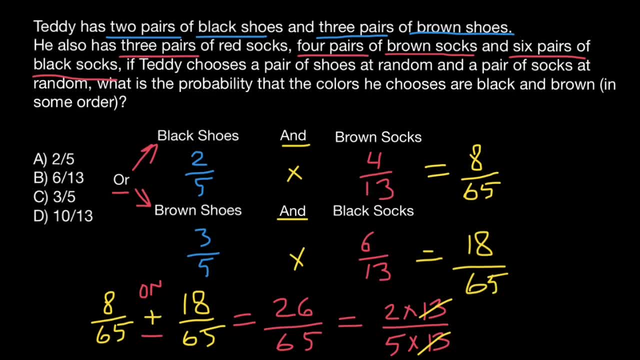 can reduce same numbers in the nominator and denominator and we are going to get to over 5 or 2 kids. as you see, this is answer. a one more time: when we connect to an independent random variable, we get 8 probabilities with the word and we have to multiply such probabilities when we 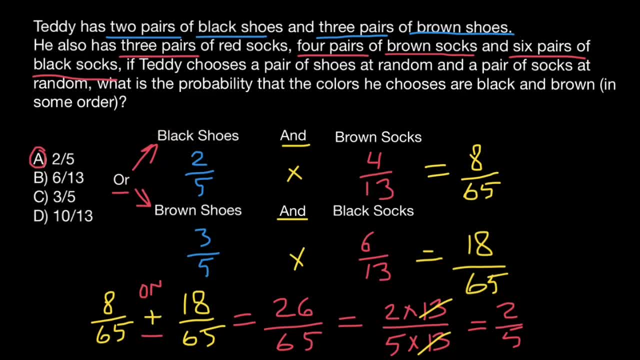 can connect to independent probabilities or set of independent probabilities with the word, or we have to add such probabilities, so we have to use some rule in this case. and this is all for today. subscribe and see in the next video. goodbye.